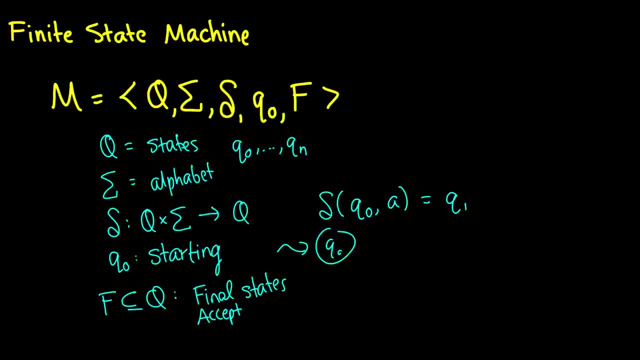 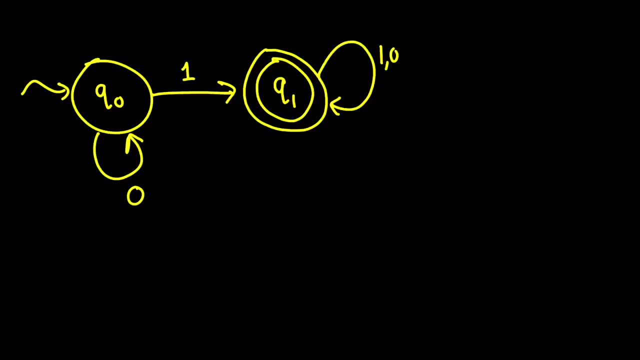 So if a machine takes you to a final state, then the machine accepts that state And it says, okay, that is a valid string of characters. So let's do an example here. This is an example finite state machine. It looks kind of nice. 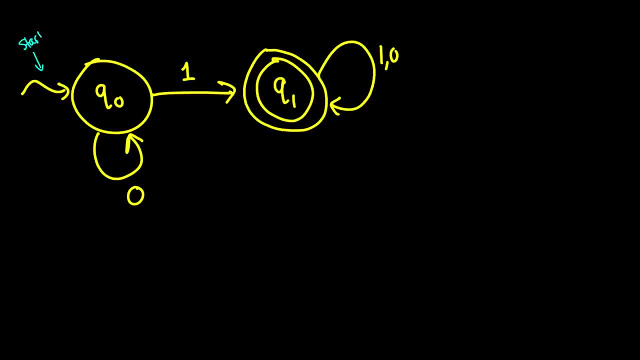 We have a starting point which is represented by this arrow, So this is where we start at Q0.. And what it does is we input a string of characters And if we give it, say, okay, we're going to let our alphabet be 0 and 1 here. 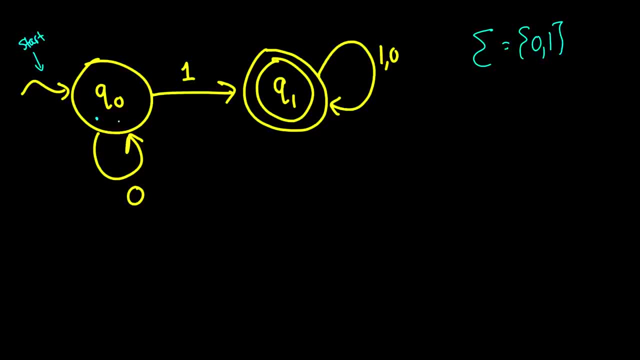 And if we give it a 0, we start in q0, and if we give it a 0, it goes back to q0.. So as an example here we'd say: delta of q0 and 0 will output q0. 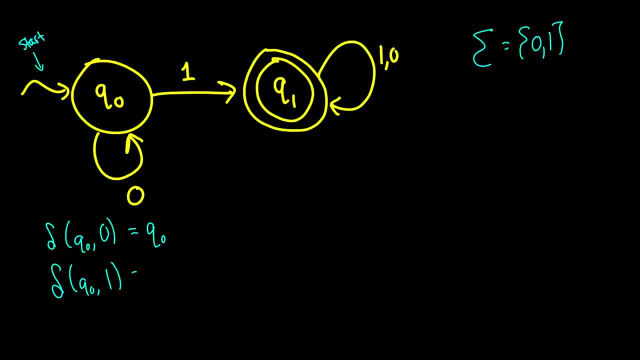 While on the other hand, if we give q0 a 1, then it goes to state 1.. So if we gave it a string, or actually, what I'll do is I'll go forward a little bit and I will denote that this q1 here, if it has a double circle around it, it is an end state. 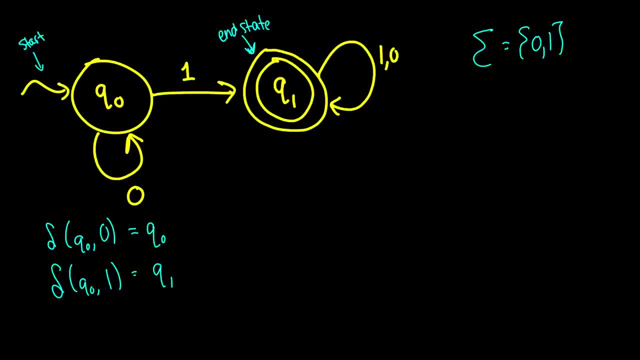 More than one state can have double circles around it, but basically the double circle means it accepts it. So if I gave a string- 0, 0,, 0, 0, and input it into the machine, what we'd say is that it's going to accept it. 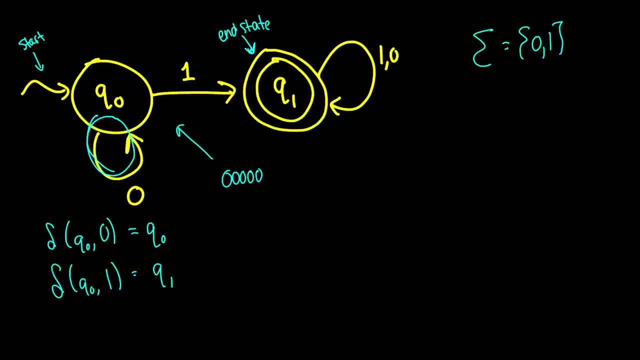 So what we'd see here is we'd start here, we'd go back to q0, then go back to q0 again, go back, go back, go back, and we'd finish in a state that does not accept it. So the character would be invalid and the language would say: no, we don't want that. 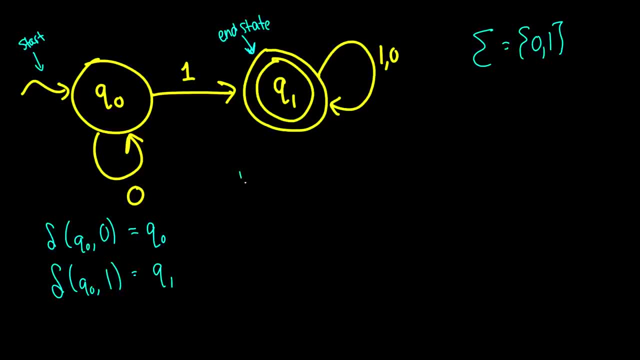 So we try again and we input the character 1.. We just give it a 1, and if we just give it a 1, the machine says okay, we finish. So we put in q1, and that is an acceptable state. 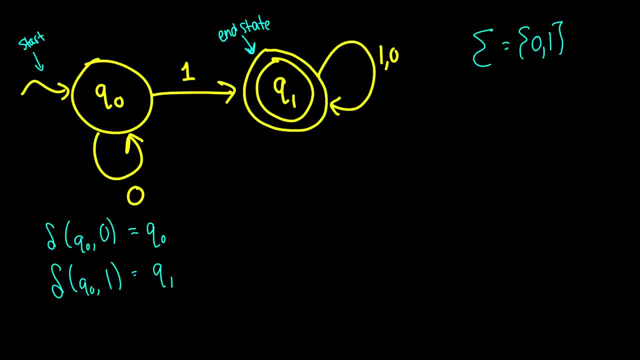 What's interesting about this machine is that as soon as you enter q1,, whatever number you put in afterwards, it just accepts it. So as long as there is a 1 somewhere in your string, the machine will accept it, And that is an interesting result, because why would you want a machine that just accepts anything that has a 1?? 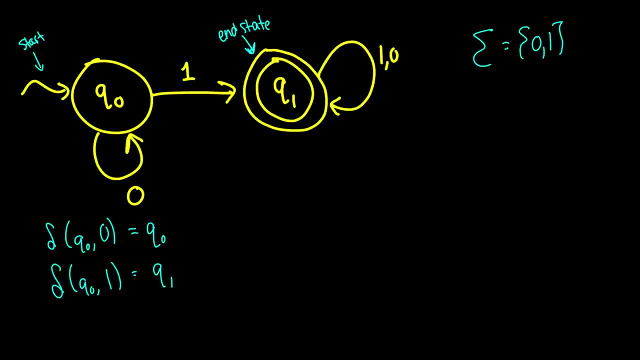 Well, if we abstract it and say: what are the applications? What are the applications of a machine that accepts any input, that is a 1?? So say there's two inputs and we say this is a yes or no. If there is at least a yes, at least one yes, it accepts it. 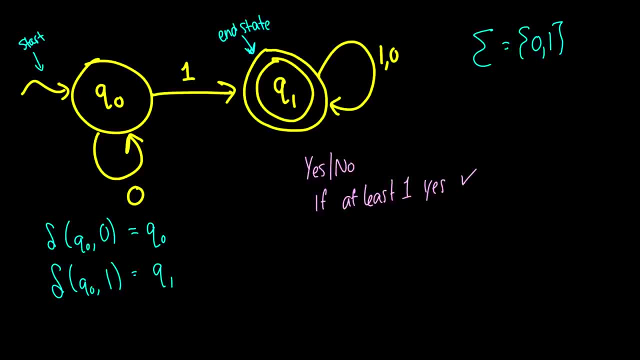 So what could you model in the real world after this? Well, perhaps I don't know. So let's say you have a program And what it wants is: it is a test program, It is for teachers and you have a student. 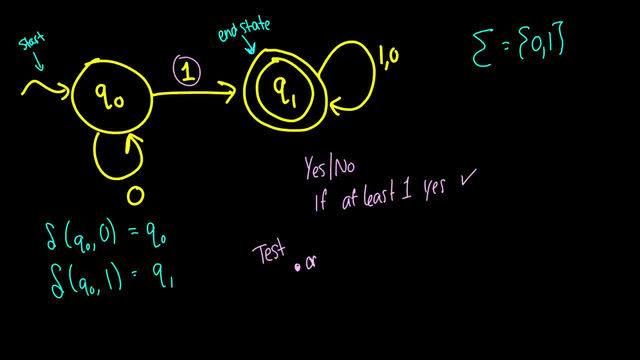 And basically, with this 1 here it's a create a student button And as soon as you press that button you have started the program And it doesn't matter what button you press after that, because that student is created and therefore you have satisfied the goal of. 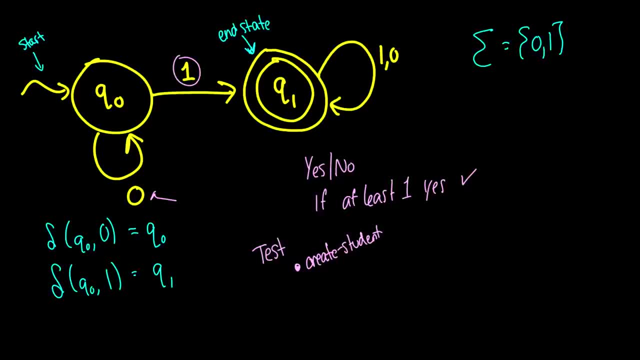 of creating a student, And here it is just not pressing any button. So basically, as soon as you open the program, you've created a student and that is your success story for this finite state machine. So a lot of these are really abstract. 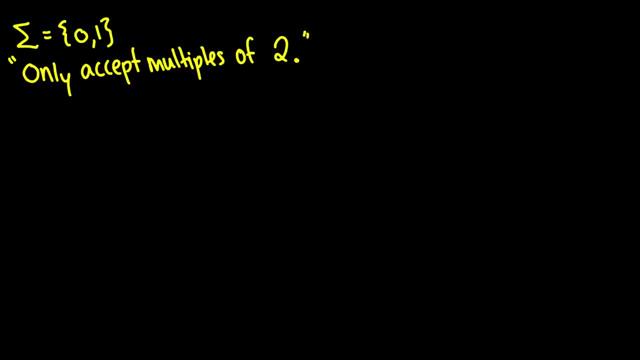 So let's get into, perhaps, drawing a finite state machine, which is something that is always fun to do, And we're given that the alphabet is just zeros and ones, and we're told to draw a state machine that only accepts multiple states. 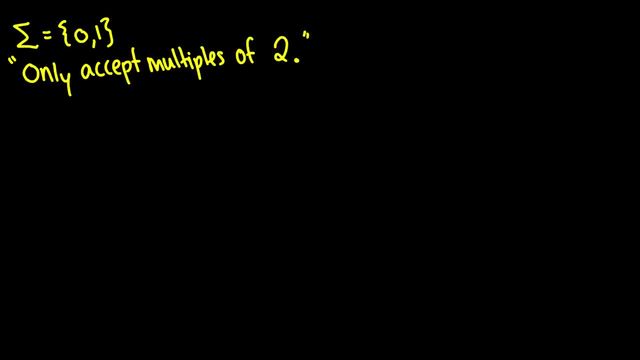 So we're given that the alphabet is just zeros and ones, and we're told to draw a state machine that only accepts multiples of two. Now here's a question: What does this mean? multiples of two? Because all we can do here are input strings like 0, 1, 1, 0, 1, 0, 1.. 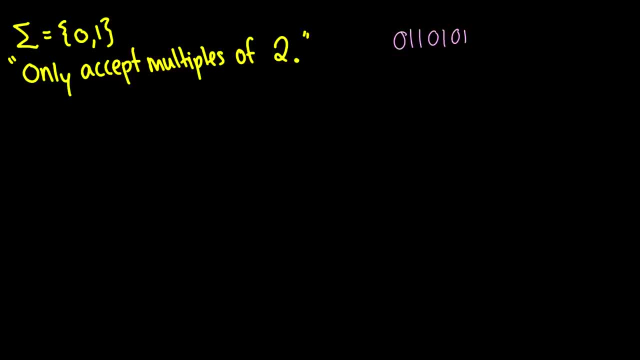 Like we can put in random strings like that. So when it says only accept multiples of two, you have to kind of abstract an idea and say, okay, what this machine really is is, if we input a string like this, what we're. 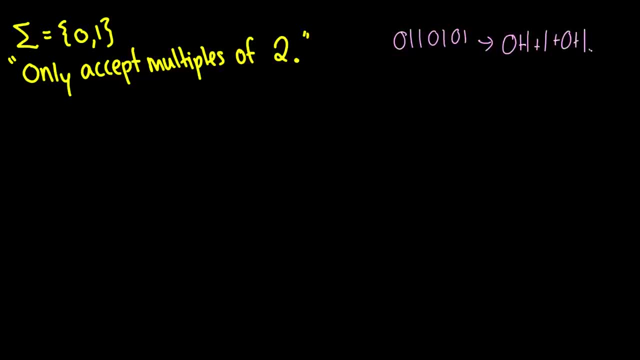 really saying is 0 plus 1.. Plus 1, plus 1, plus 0, plus 1, so on and so forth. So you have to sort of define what you're doing, because finite state machines are actually more abstract machines that you apply to things. 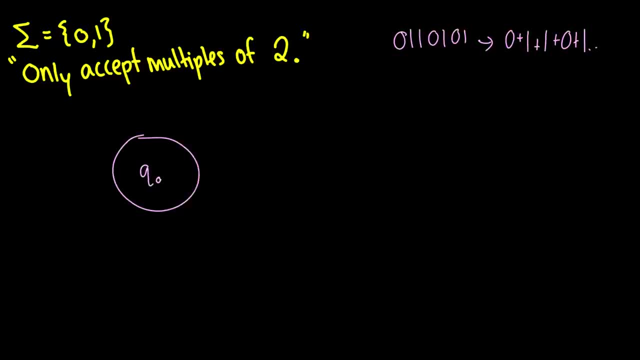 So what we do is we start out with an initial state. we'll call this q0, we'll draw a little line to it, and it only accepts multiples of two. So let's think of some strings that it would accept. Let's think of some strings that it would accept. 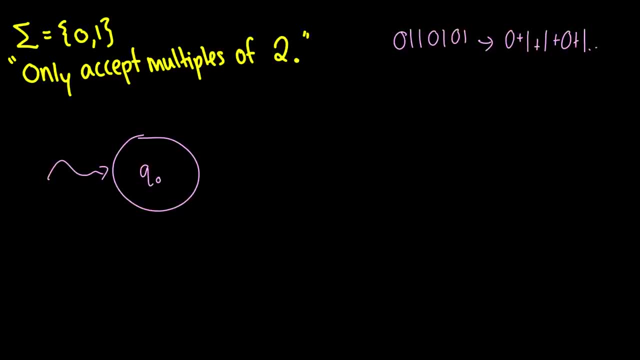 Let's think of the most bare minimum strings it would accept. It accepts the state. I'll do this in green. it accepts 0.. It accepts 1, 1.. It accepts 0, 1, 1, 1, 0, 1, 1, 1, 0.. 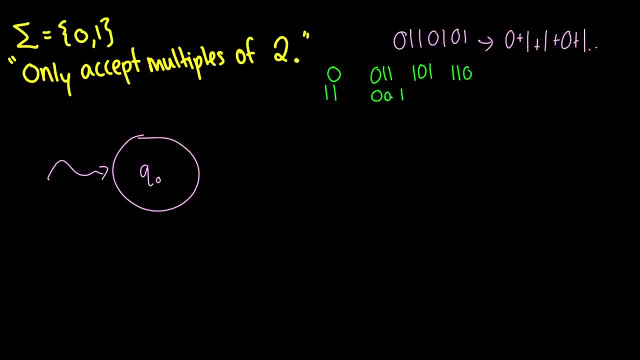 It will accept 0, 0, 1, 1.. Now, we've done a lot of things it accepts. What about the things it doesn't accept? And this is equally as important. So these are the okay boxes. Now the bad boxes are 0, 1, 1, 0, 1, 0, 0, 1, so on and so forth. 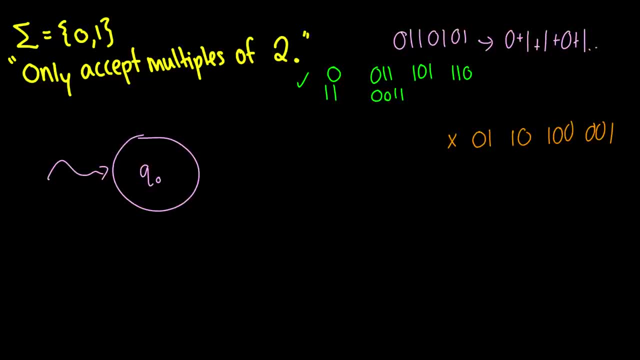 So the question is: how do we start? Well, if we don't do anything, and even if we just have, say, an empty string, that is also acceptable- then we're going to start off in this state here And it's going to be accepted. 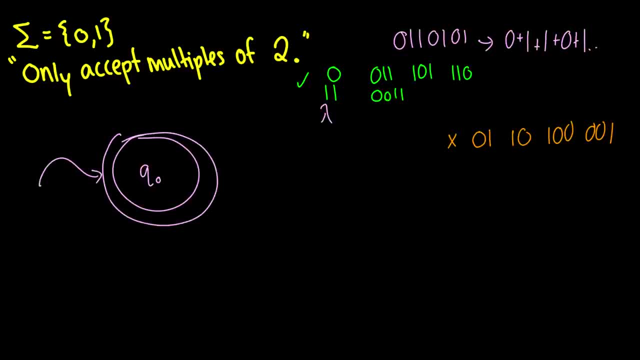 As soon as you start the machine it is accepted. So because the empty string is an accepted final state, the first one is accepted. Now here's the thing: because there are clearly things that aren't accepted, we have to draw another state over here, q1,, that doesn't accept things. 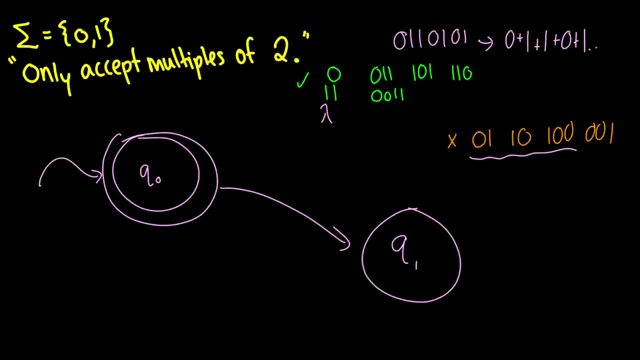 And how does it not accept things? Well, here's the thing: If you just input a 0, you're good in the first state, But as soon as you put a 1 in, it goes to this not accepted state. Now here's the question is: how do we get back? 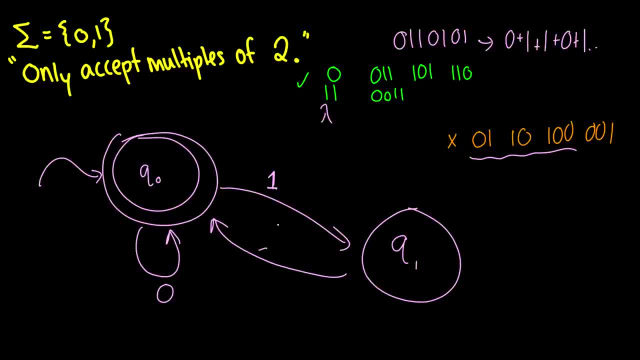 Well, if we put in another 1, we're okay, Because, in order to have two 1s accepted, you go to q1 if you're an odd number of 1s and you go back to q0 if you're an even number. 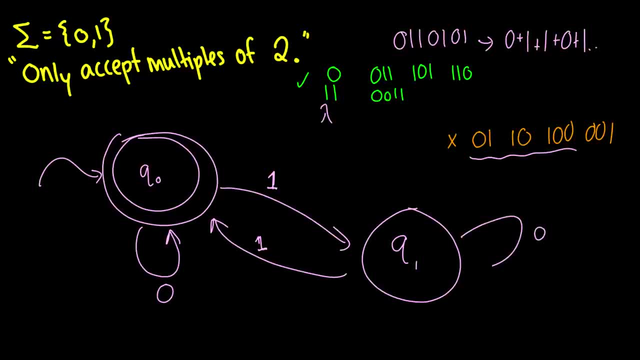 And then you go to q1 if you're an odd number of 1s, and you go back to q0 if you're an even number And clearly 0s don't have any effect on the machine whatsoever. It does not take a state from one to another. 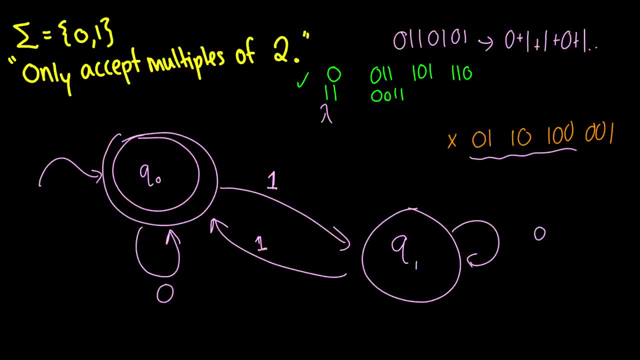 Because you're adding 0s, you're effectively doing nothing. So we have these 1s alternating states back and forth. so when there's an even number of 1s, it's in q0, and when there's an odd number of 1s it's in q1.. 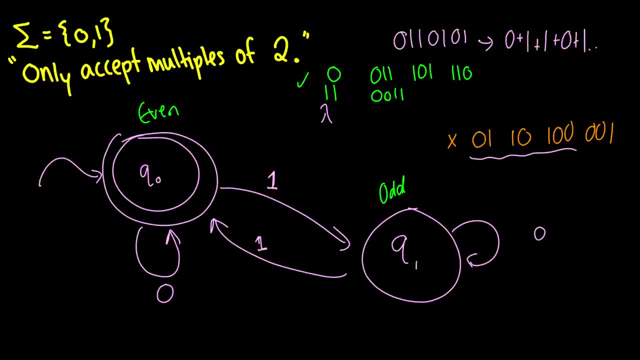 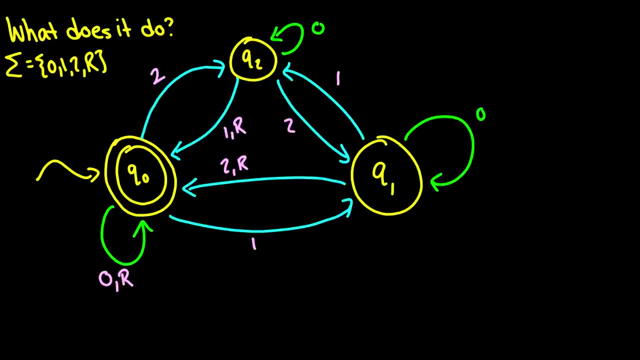 And that is a finite state machine that accepts multiples of 2, given this alphabet. So that's pretty cool All right, now that we know how to draw them. what about if I give you a state machine and say, what does it do? 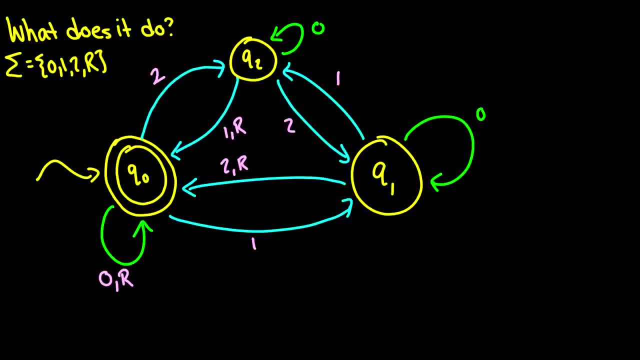 In fact I've been a little vague here. I've said: well, sigma is 0,, 1,, 2, and the letter R. What does R stand for? Well, you've got to figure that out. So take a moment, look at this machine and tell me what you think it does. 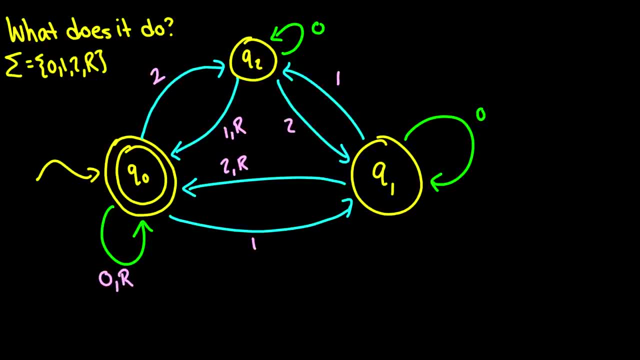 All right, hopefully you've had a look at this. So here's the thing: The first machine, the first state, it just accepts. It says OK, that's cool. So if we take the string 0, it accepts it. 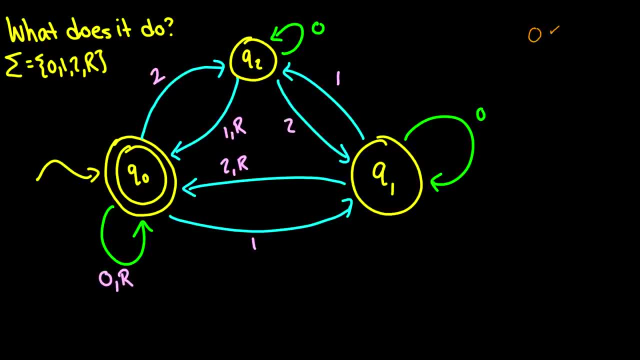 Cool. Now what I notice here is that it also accepts R. In fact, if you take a look at this very closely, it looks like no matter where you are- say, if you're at q2 and you input an R, it accepts it. 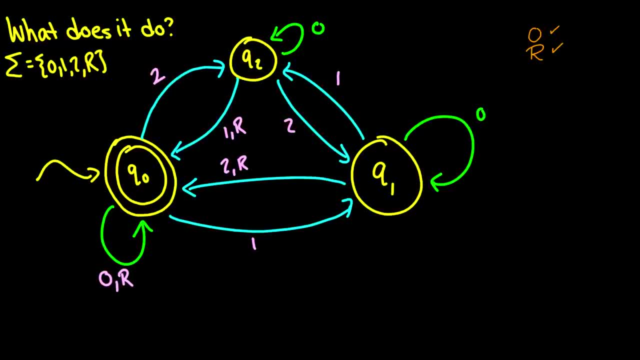 If you're at q1 and you input an R, it accepts it. So basically, anything that ends in an R, it also accepts. So we can kind of think, OK, maybe this R actually just means reset. That's probably why it shows R. In fact, in the original example the word was reset. 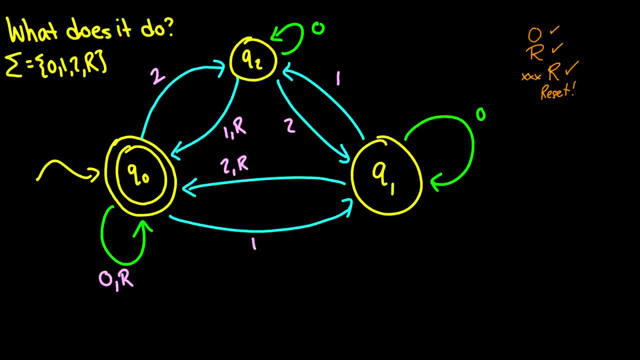 I was just being mean by taking out the letters ESET, But OK, so that's kind of interesting. If it resets the machine, it's OK. If it's a 0, it accepts. Now what does it do here? 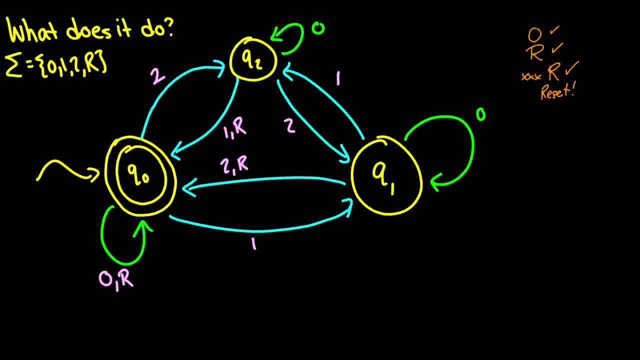 Well, perhaps it's an addition convention that we've done before. So let's take a look at some strings. Let's say, OK, if we put in a 1, then we go from q0 to q1.. And then if we put in another 1, we go to q2.. 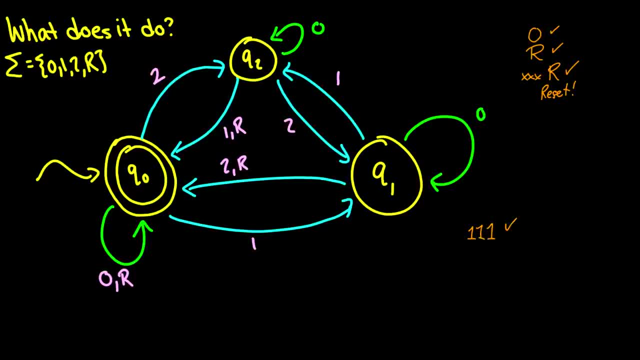 And if we put in another 1, then that's OK. OK, Let's do something a little bit different. Let's traverse to q1 and get back to q0.. And we can do that by putting in 1 and 2.. 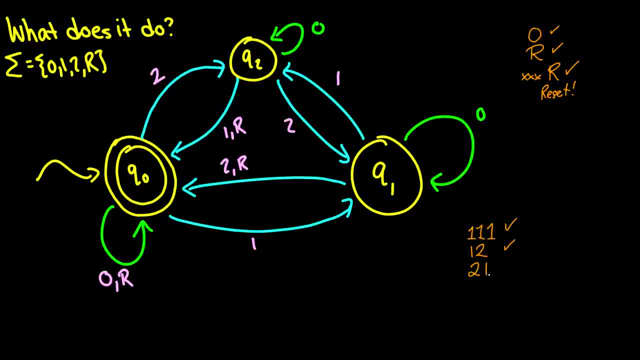 OK, What if we want to go to q2 and then back to q1? We can put in 2, 1.. Hmm, It's kind of interesting. But what we haven't done is we haven't gone from q0 to q2, to q1 and back. 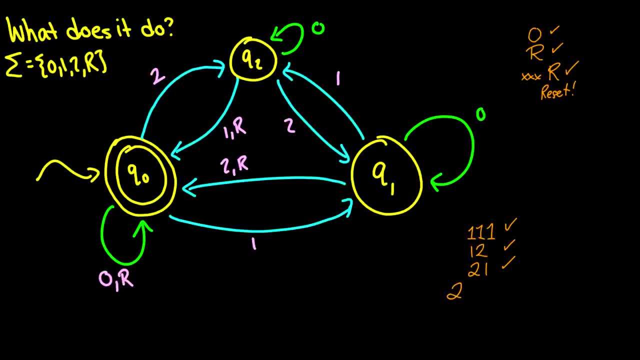 So let's do that path, OK. Well, from q0 to q2, we can do 2.. From q2 to q1, we can do 2.. And from q1 to q0, we can do 2.. 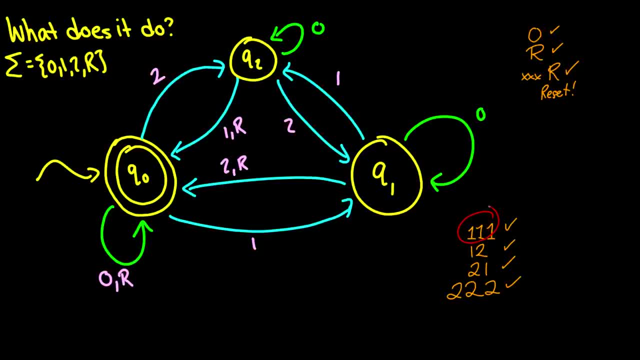 And that's OK. So what we kind of see here is that if we add these numbers, they all equal 3.. So we can kind of assume that, hey, as long as our string equals 3, it accepts it. And just to test this, let's put in: 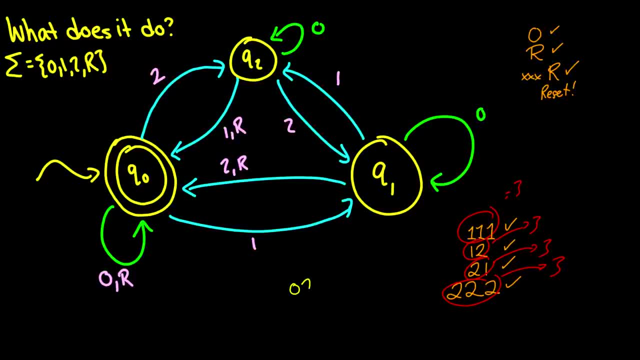 Let's create a string in our head, just a random one: 2, 0, 2, 1, 0, 0, r. 1, 0, 2, 0, 1, 2.. 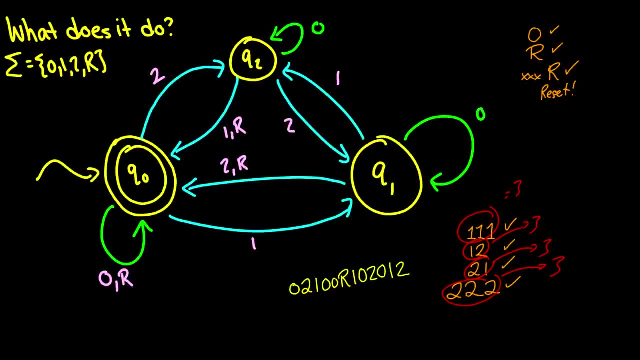 And according to this string, this should accept. So we just randomly pick some numbers. Now, if we follow the machine, which I will do in dark purple and then erase afterwards, we start. It's not a good color to do this in. 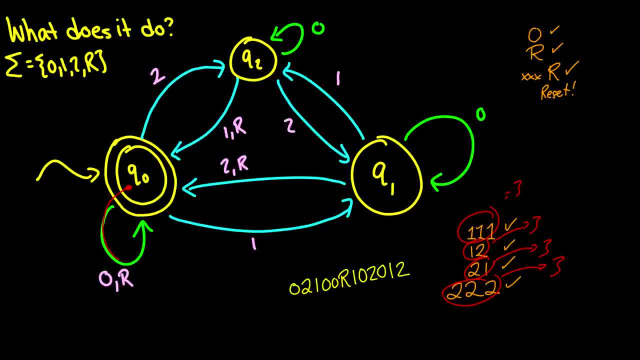 Let's do red. So we start with q0. And we do 0, so we go here. We do 2, so we go to q2.. We take a 1 back to q0. Then we do a 0 a couple times. 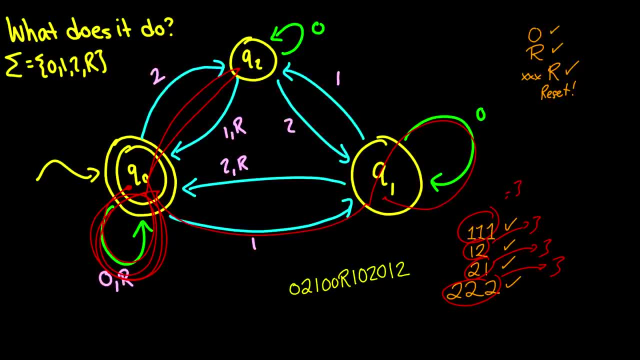 Then we reset once. so that's good. We now take a 1.. We take a 0.. We take a 2, which takes us back to q0.. We do a 0.. We do a 1.. And then we do a 2 again. 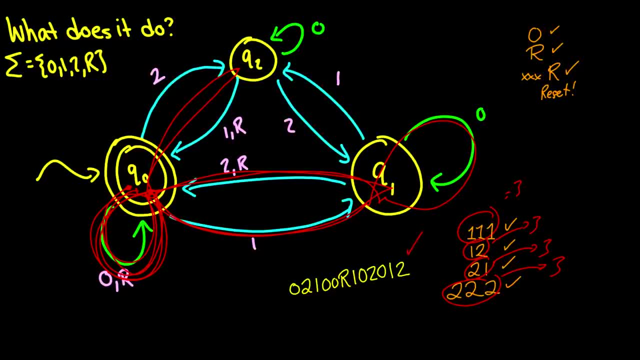 And we end up back at q0.. So it's accepted, just like our hypothesis. So it accepts multiples of 3.. Basically, what this means is that this is a 0 mod 3 check, Or I should say a 0 is equal to n mod 3 check. 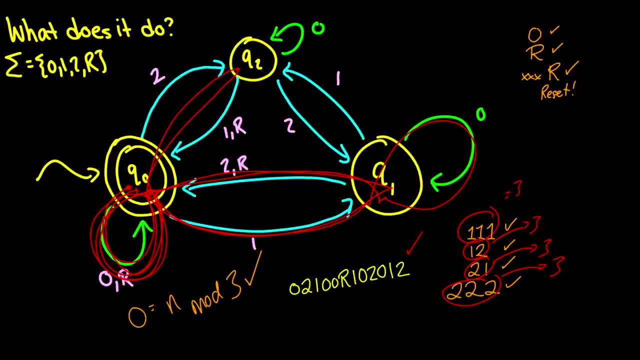 And if this is the case, it accepts it, If not, it rejects it. So you can play around with this. You can make sure, hey, after the last reset, our string adds up to a multiple of 3. And if it does, then it accepts the machine. 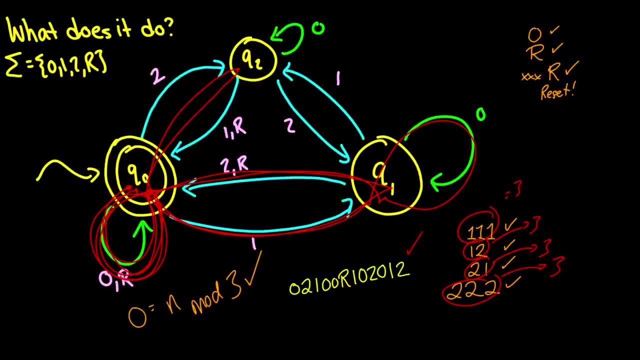 And you can play around with this. So that's kind of cool. And that is the basics of finite state machines. You can do crazy things with them. You can construct a machine where, in fact, it only takes multiples of 7.. 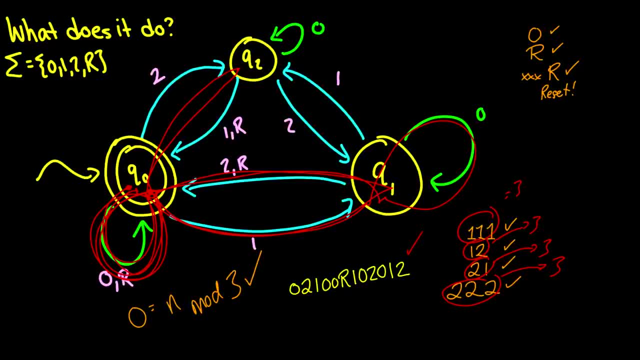 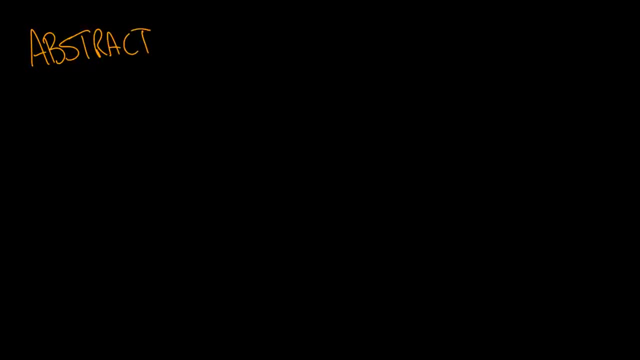 Or maybe any string that has common factors Of, say, 2 and 5. Which, again, these are really complicated machines compared to this, But they can be done. And the main important part, which I didn't write anywhere, is that these are abstract. 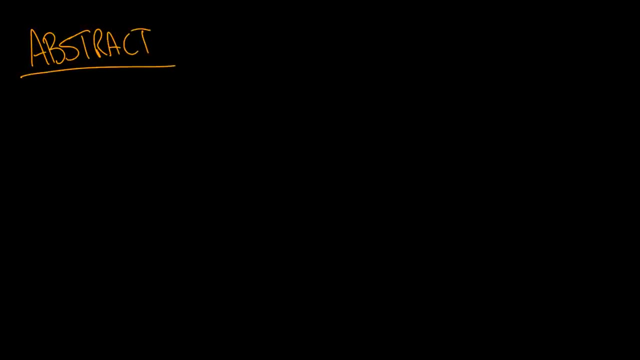 Of course, these can be very concrete and just be drawn to do what you want, But most of these are sort of like programming flowcharts, And I think that's probably the best way to describe this Is that these are flowcharts for your programs or for operators. 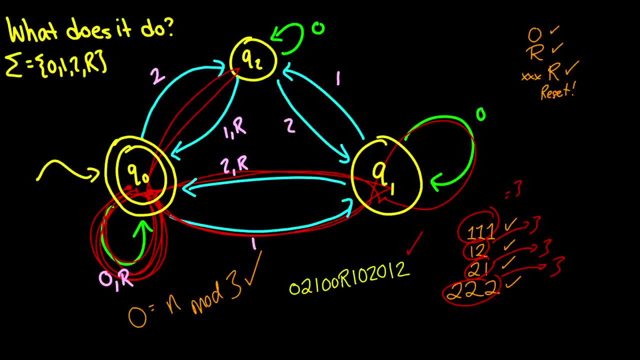 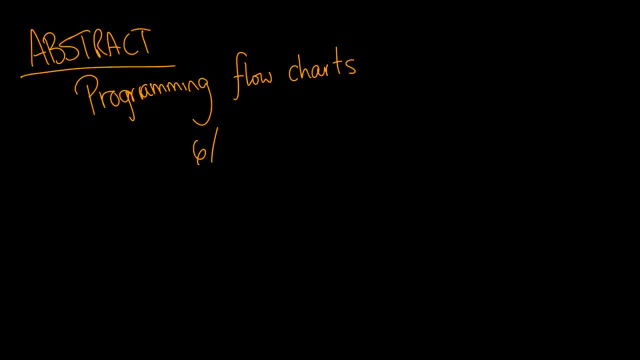 For instance, this 0 mod 3 check is kind of an algorithm, right, Because it takes a number and then it does a bunch of things and keeps It, basically subtracts 3 times n and checks: okay, does it equal 0?? 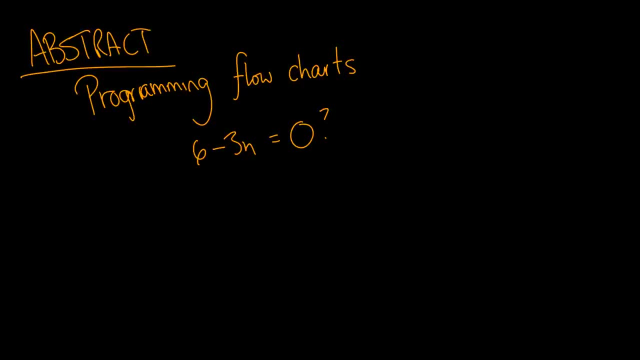 Well, yeah, it does, So it accepts it, And you can do this for say: okay, well, What if, instead of this sort of thing, we have 3 different types of numbers, Let's say we have odd numbers, we have even numbers. 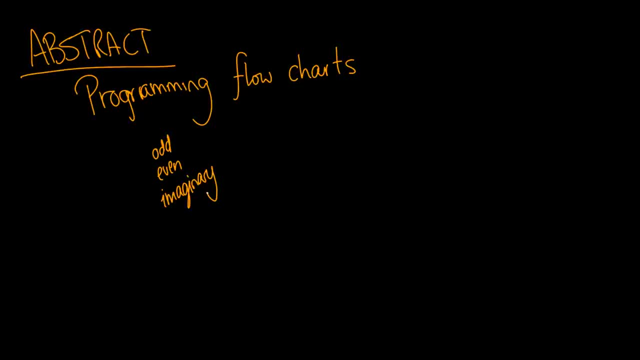 And then we have these imaginary numbers which are neither odd or even. I'm inventing something here. So we'll call these, We'll draw the numbers like this: It's just an imaginary number And it's like an x with two dots. 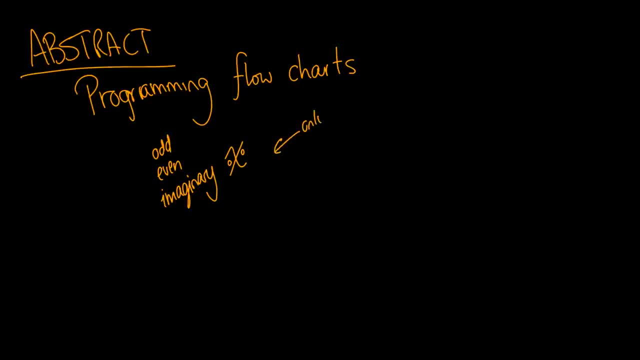 We're doing this and we say, okay, well, I want a machine that only accepts these. So basically, it only accepts these, And there's certain combinations of odd and even numbers that you can make with this cool operator that is a donut with blazing suns coming out of it. 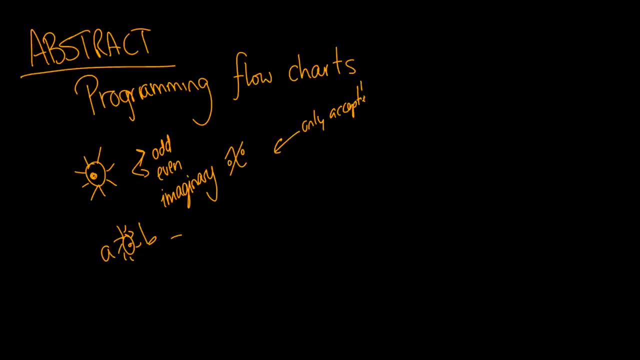 So if you take a and you have this little star thing, b, then you can get this imaginary number out of it, And this is really abstract and crazy, right? But you can design a machine that, under specific circumstances, does this And then you can program it. 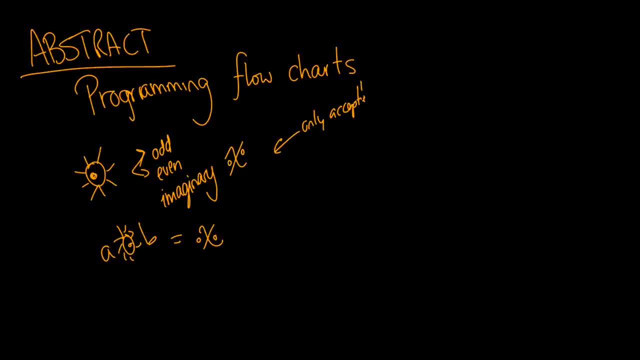 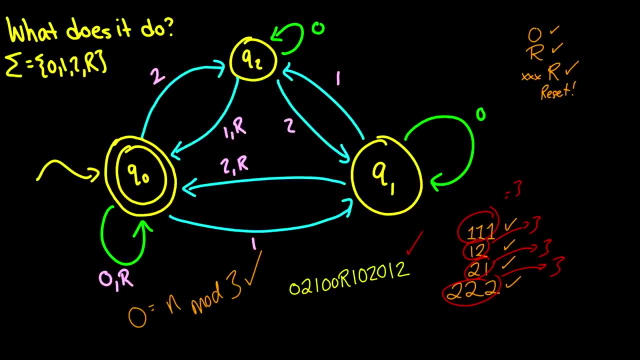 So that is the whole purpose of finite state machines. Clearly things you would talk about in a formal languages course or further mathematics. I will erase this red line. So here we see that if we start at q0,, we put in 0, we go back. 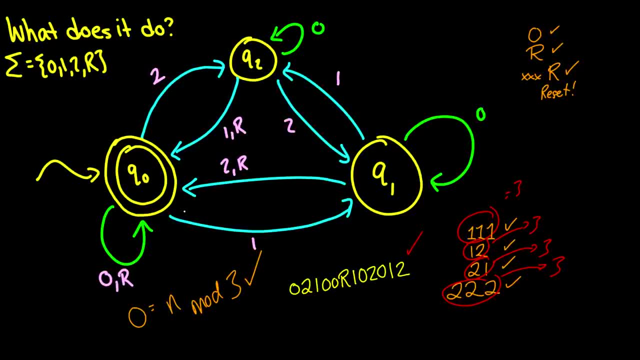 We put in r, we go back. If we put in a 2, we go to q2.. If we put in a 1, we go to q1.. It is pretty deterministic, Like we know where we're going. 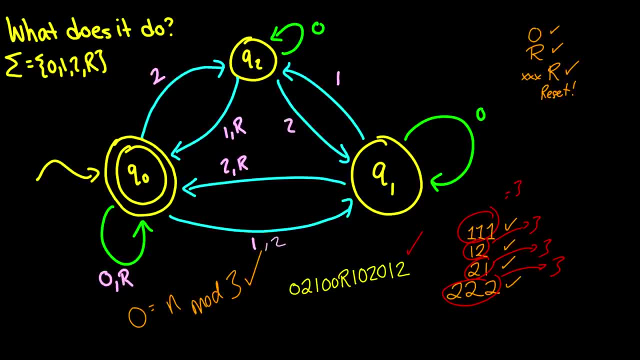 But what if I said, okay, if you put in a 2, you might go to q1 as well. instead, If you're in q1 and you put in a reset, well, you might go to q2.. In fact, you might even just go back to itself. 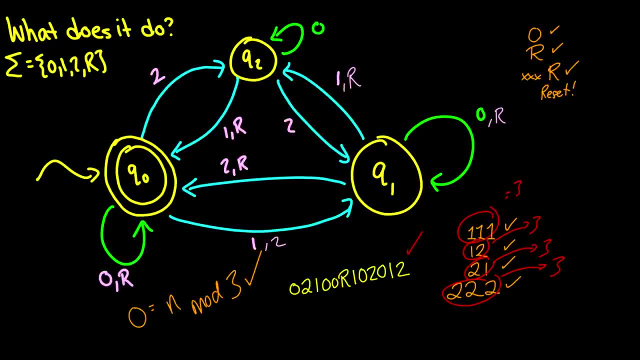 Who knows? And what about from q2?? Well, basically, anywhere you go, it may be a 1.. It would be nice to go back to itself too. And then you have a non-deterministic finite state machine, And that gets a little bit more interesting. 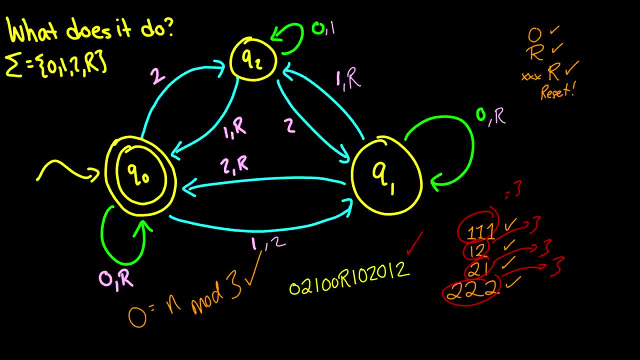 But if you're interested in that, there is tons of stuff online. That was finite state machines. If you have any questions or good homework problems, that you should probably let me do on camera, because a lot of homework problems in discrete math they don't really touch on finite state machines. 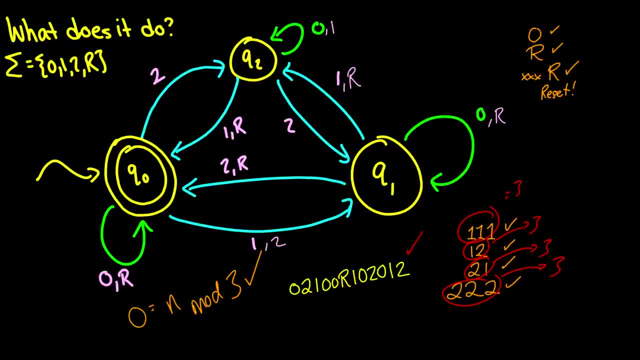 And if they do, they usually go a little bit beyond this And that's normally not taught in the first course, But I'm including it here. so kind of a weird spot to be including this video. But if you have any questions, leave them in the comments and I will answer them as quickly as possible.